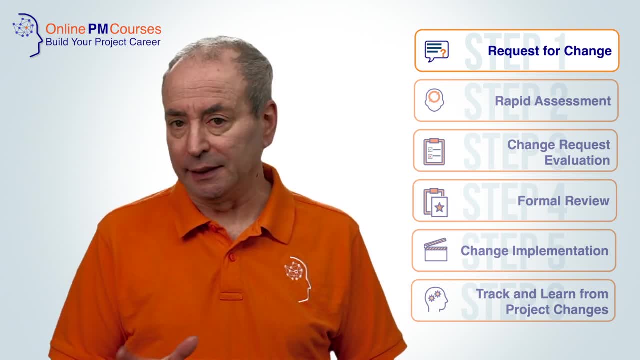 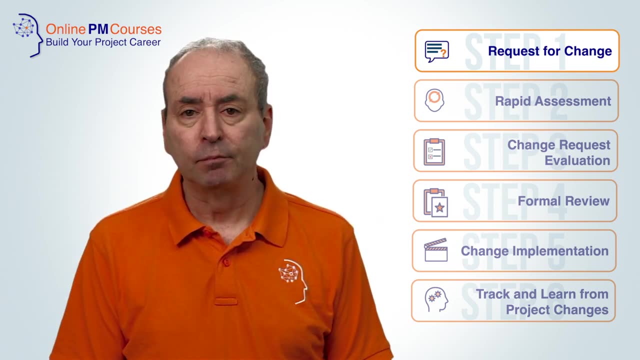 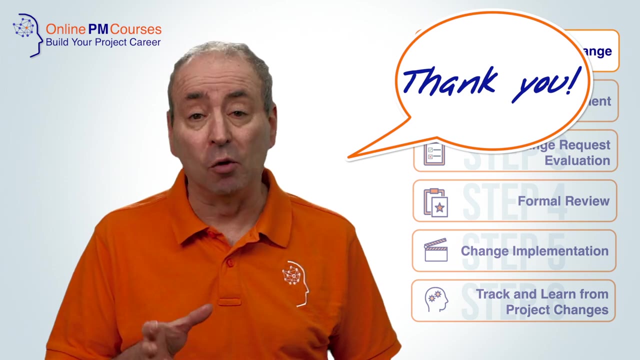 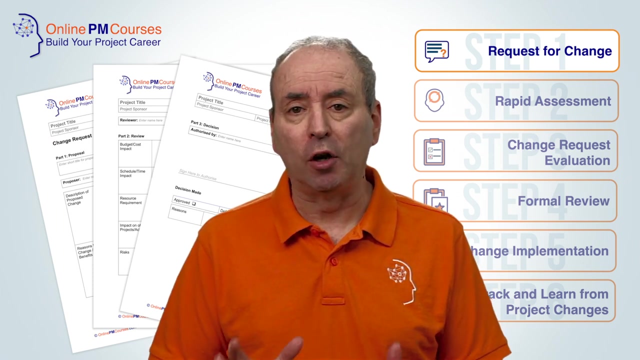 a suggestion or a request for a change. This is known as a change request, or a request for change or an RFC, Whatever you call it. your first response is simple: You thank them for their suggestion or their request and you take note of it. You'll need a simple change request form to document their request. 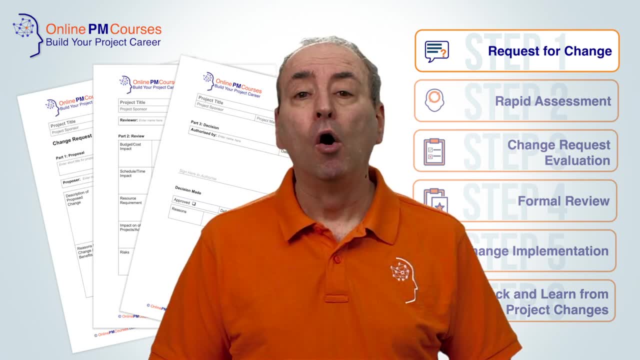 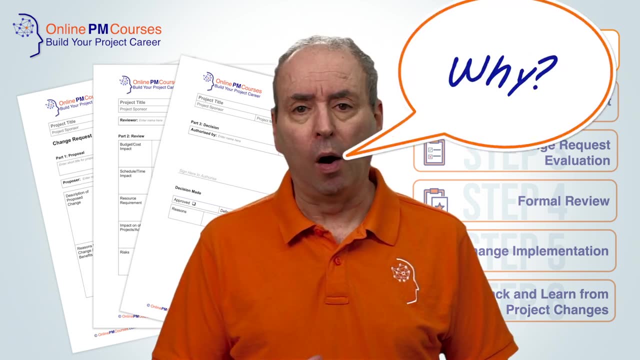 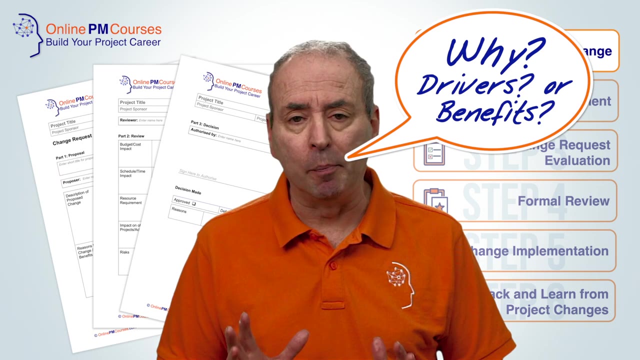 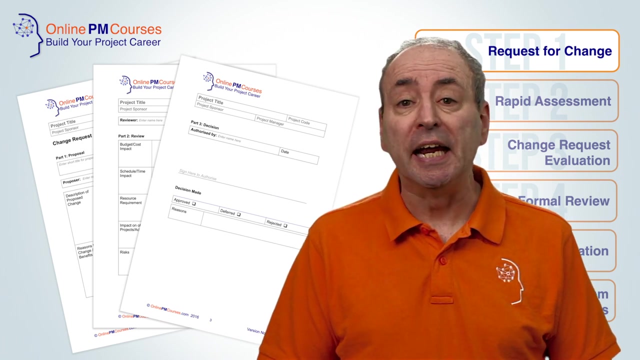 And the most important questions to ask them are: what precisely is the change you're suggesting or recommending or requesting, and why? What are the drivers that make this change necessary Or the potential benefits that make it desirable? A change request form is likely to be structured into three parts. Part 1 is the proposal. 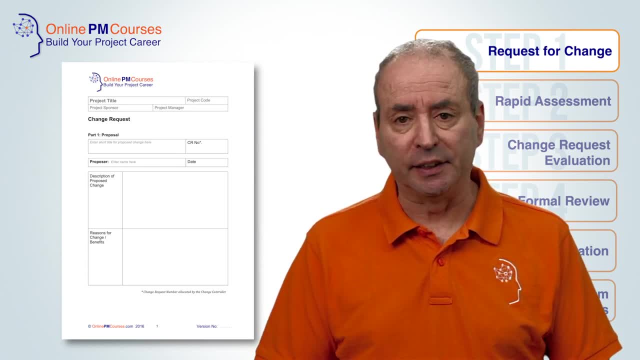 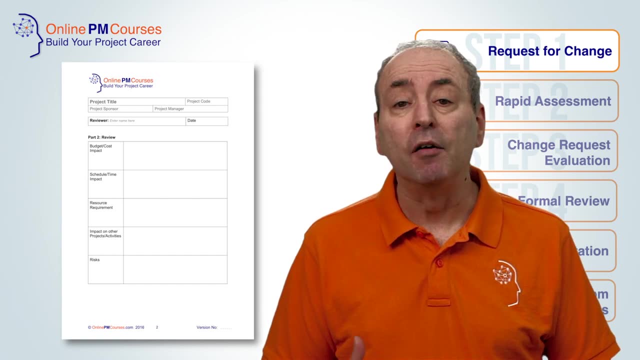 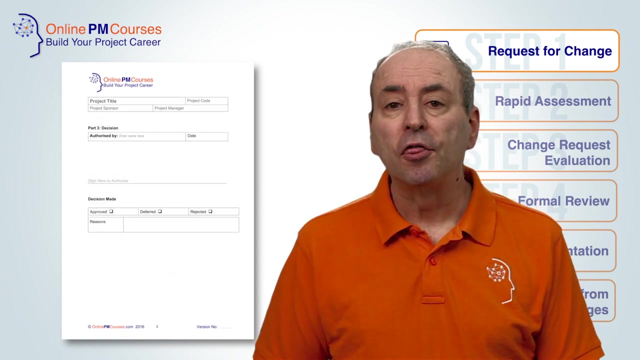 This documents the change requested and the reasons. Part 2 is the review, which documents our assessment of the implications of those changes, which we'll talk about more at stage 3.. The third part is for the decision. This is where the decision maker, or the decision makers, 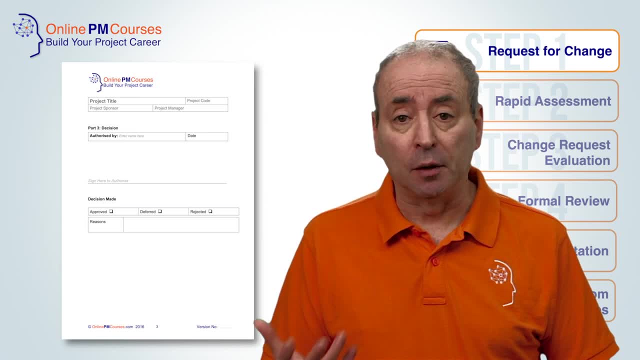 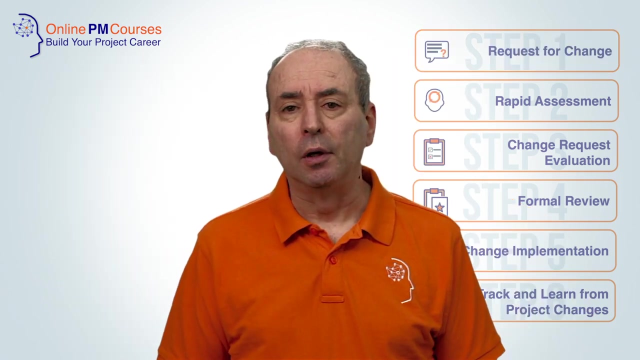 will record their decision, either to support and uphold the request or to reject it, and, importantly, their reasons, And it's usually accompanied by some form of endorsement in the form of a signature. Step 2. Change control- rapid assessment. Not all change control processes will. 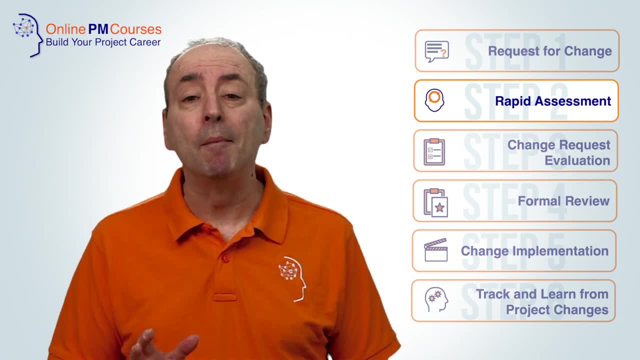 have this step, but to me it makes sense for the project manager to conduct a rapid assessment of the change request. There are two things that I would typically consider at this step, And the first is my familiarity with the change requested. Has this request been made before? 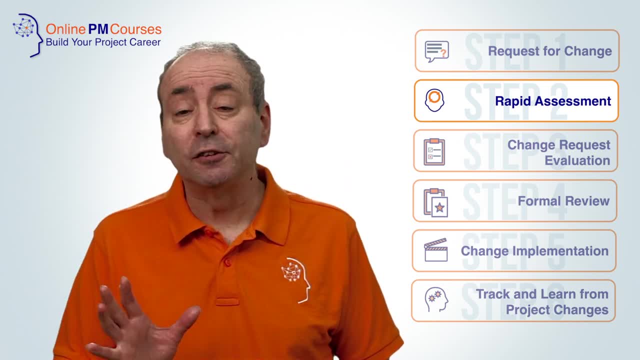 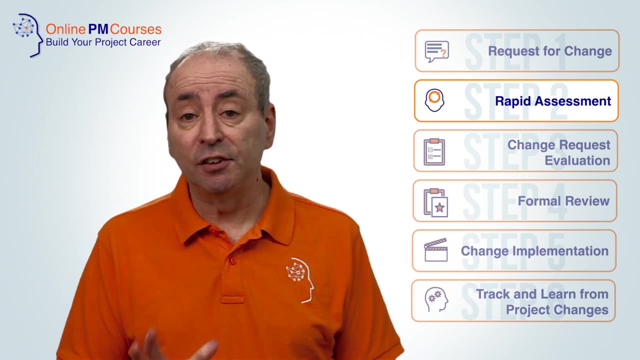 If it's new, then I can move on, If it sounds familiar, if it's the same as or similar to one that's already been requested, has a decision already been made? If so, I'll let the requester know And I probably won't need to take any further action. 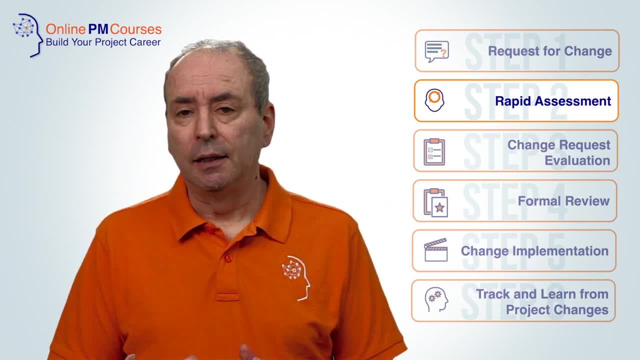 If the change request is still in progress, then does it make sense to combine the existing change request with this new one? Does this new one add anything to it or does it modify it in any way? that is material that I need to take into account. The second thing: 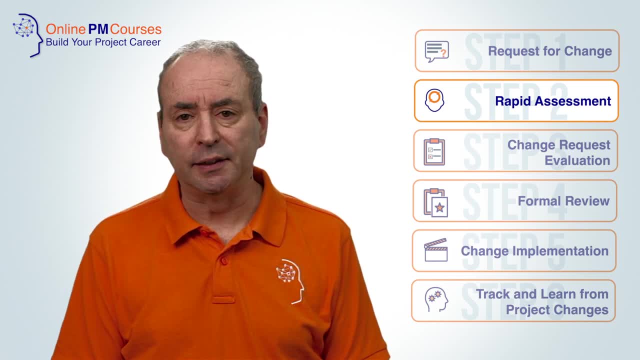 to consider is the scale of the change request requested. In some contexts, the project manager will have the authority to deal with minor change requests on their own, to evaluate them and to make their decision. This will usually be based on their seniority within the organization. 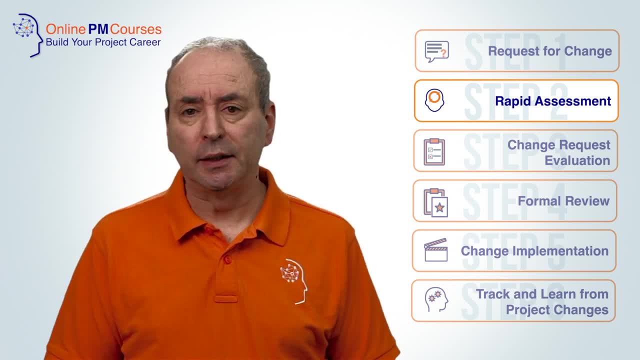 So ask the question: does this change request have either a nil or a small impact on the schedule, the budget, the resources, the risk or quality of the project? If so, it's likely that you, as project manager, will be able to make a decision with minimal formality. 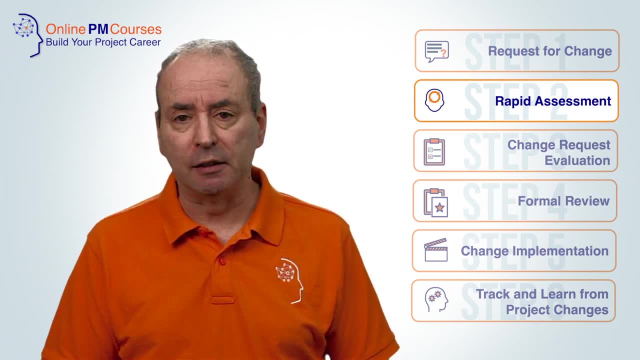 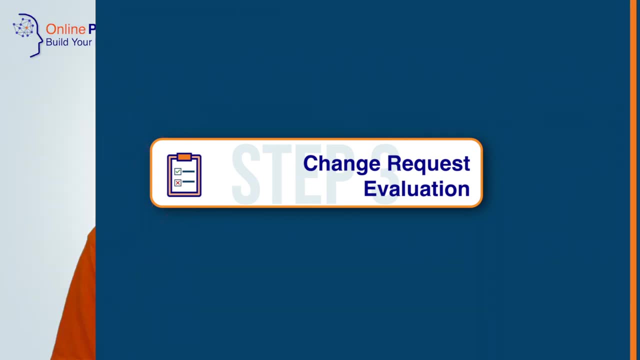 It doesn't, however, mean that you shouldn't be recording the change request and your decision. Step 3: change request evaluation. The bulk of your work will depend on your decision making. The bulk of your work will depend on your decision-making process. I have faith that your decision will come at this step. 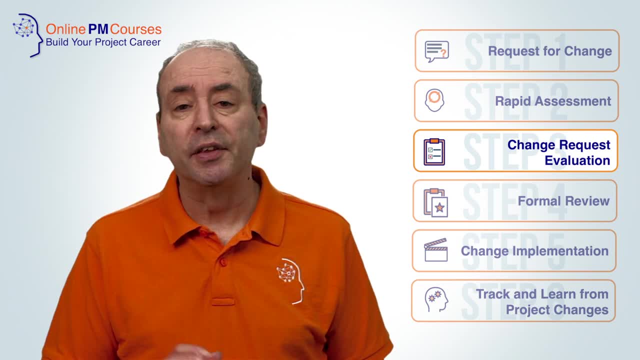 Work with your team to document the implications of the change requested for things like the project schedule, the budget, the resources you will need, the risk profile of your project and on implications, but other things that are going on around your project. This evaluation will allow you to complete. 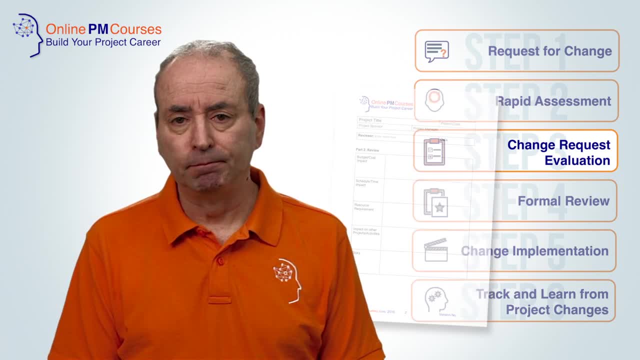 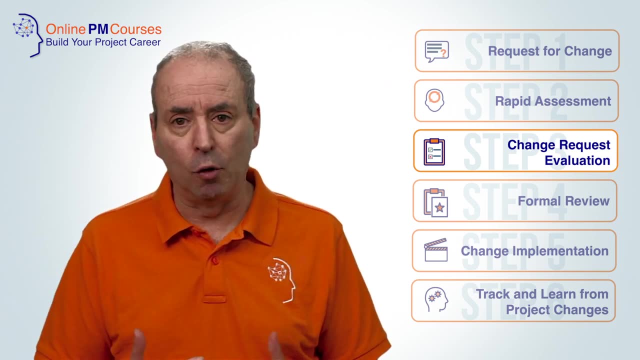 the second part of the change request form. this means you'll be able to present the decision maker- which may be an individual or it may be a change control board of some form- with a balanced argument, a mini business case which sets the benefits or the drivers for the change against all of the implications of that change, which are 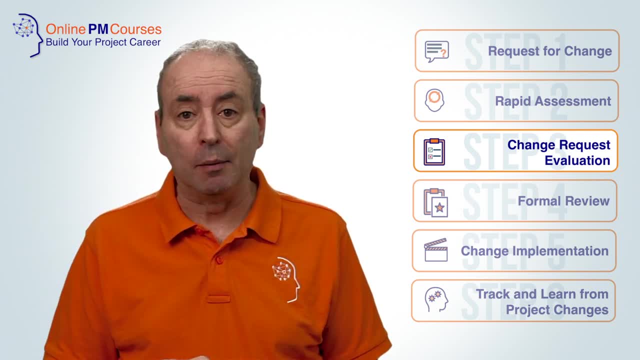 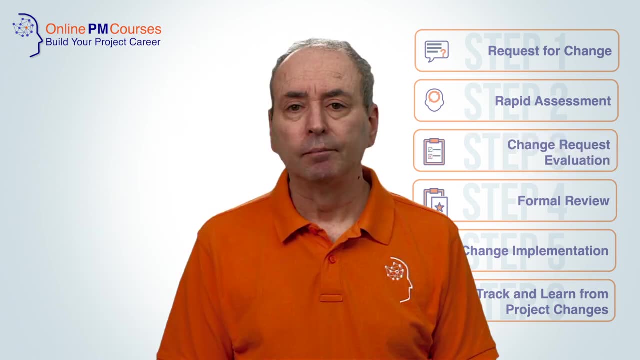 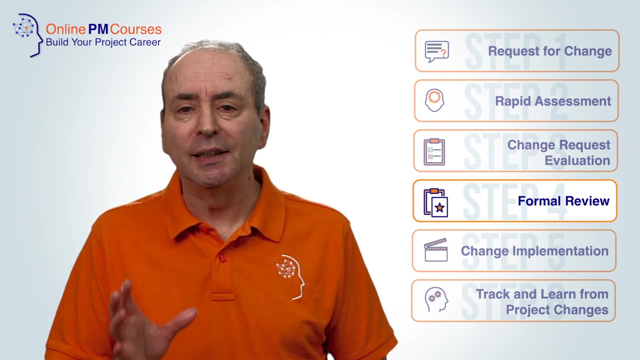 likely to be increases in the budget, the resource requirements, maybe even the risk profile and and the time it will take to deliver your project. step four: formal review your project. decision makers need to assess the case that you have put forward and, based on the evidence, they can make. 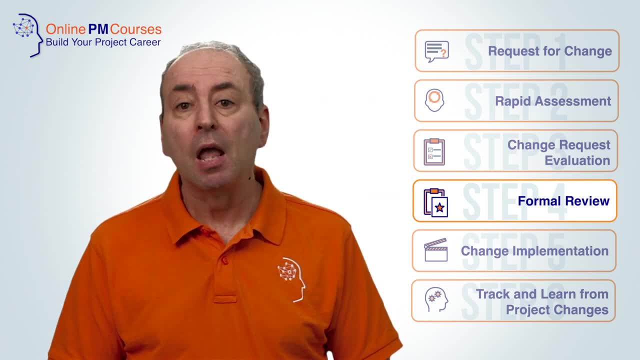 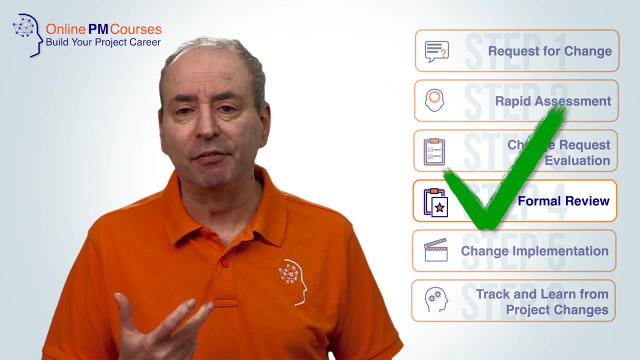 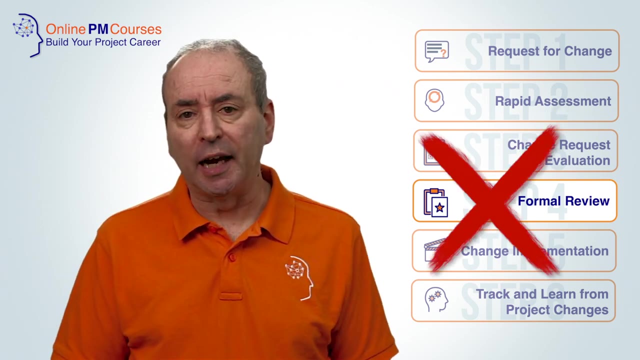 one of three possible determinations. firstly, they can choose to accept the request for change because the case is compelling. the benefits outweigh the costs and the risks you. second, they can choose to reject the request for change because the case is not compelling. the benefits do not outweigh the costs or the risks or the delays. 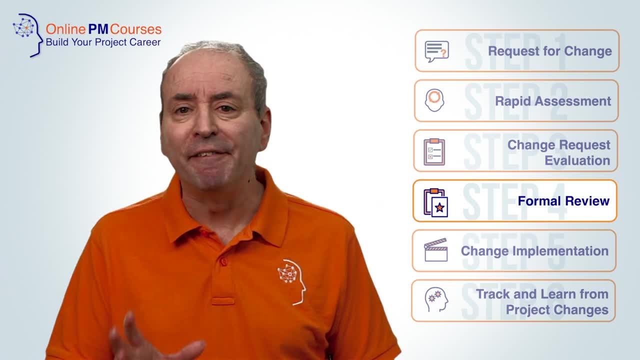 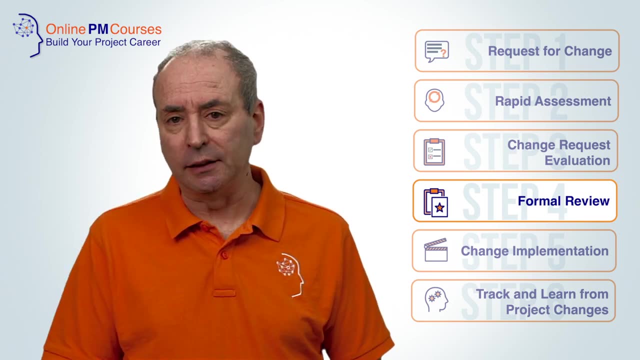 the third option is to defer their decision. however, to my mind, there can be only one reason for deferral, and that is because they do not have enough information to make a definitive decision, which raises the question: why would that happen? why would they not have enough information? 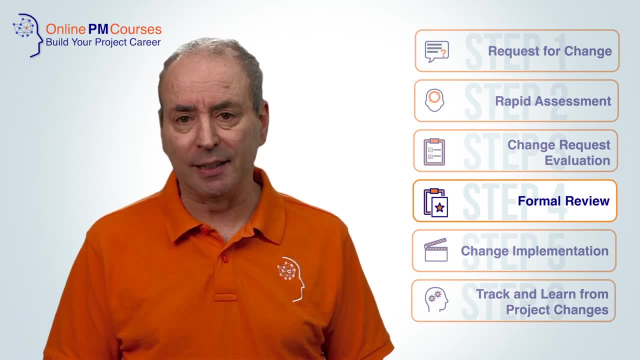 and that, my friend, is down to you as the project manager. it's your job to provide all of the information they are likely to need and to get to know their information requirements, because the implication of a deferral is that it is likely to increase the cost. 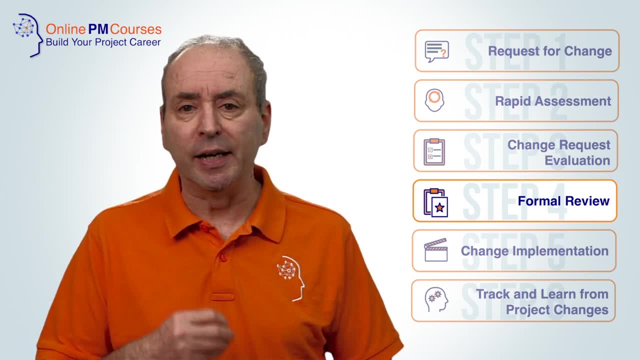 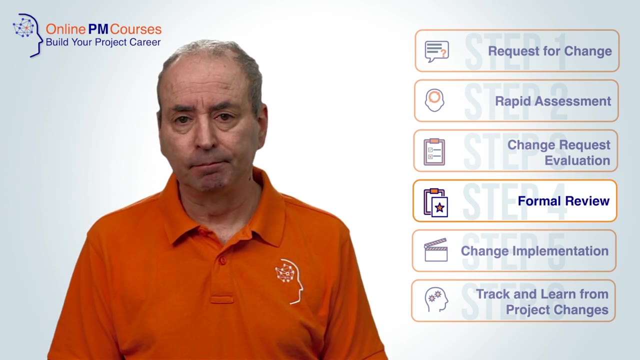 and possibly the resource requirements and the risk of making the change a deferral, should be able to make a definitive decision whether or not the project would meet. the decision maker or a change control board of any kind needs to know that it must not defer any decision unless it cannot reasonably make that decision. Step five: change implementation. 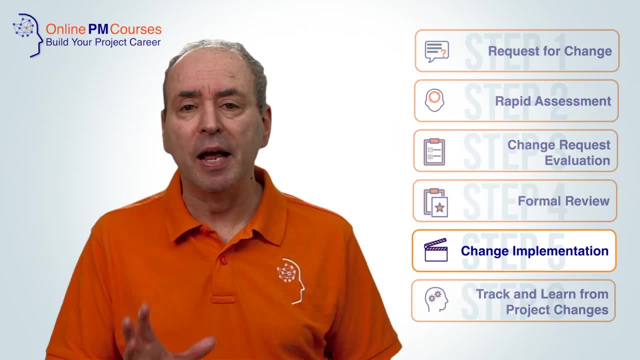 Now it's time for you and your project team to implement the change that has been accepted. Now the good news is that you've already calculated the impact on budgets and schedules and resourcing, which means you have a plan. So really it's just work. Step six: track the changes. 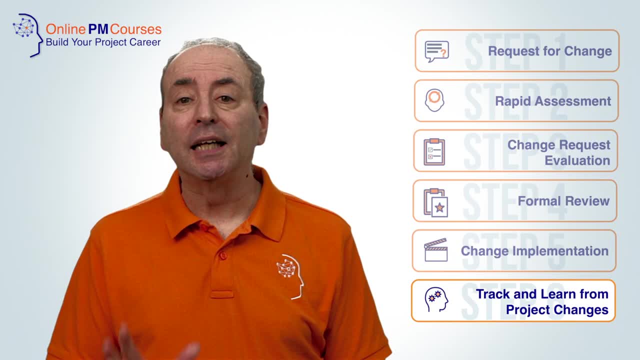 that are being made and learn from the process. As with all good project management, you need to monitor and control what is being done and learn from the changes that you make. When the changes are complete, learn from the outcomes. What was the impact of the changes? How did the process?